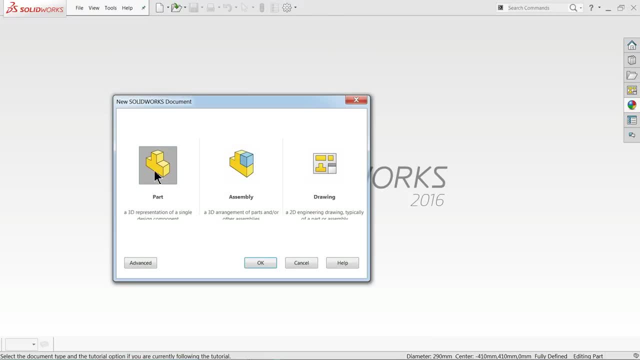 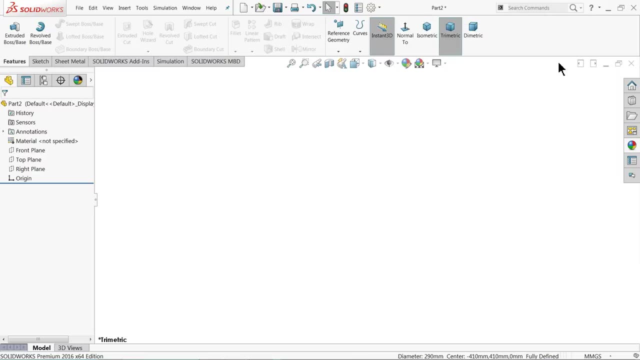 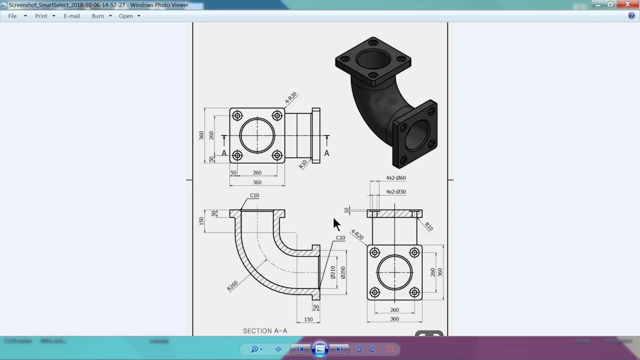 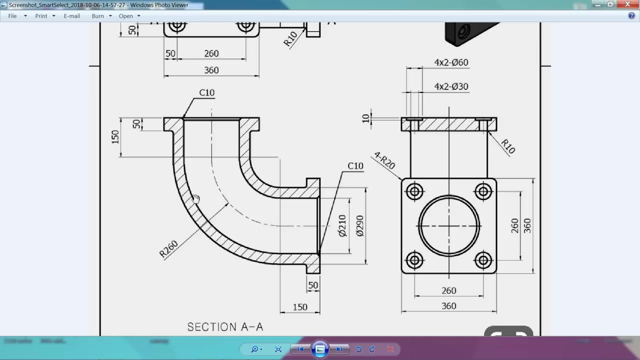 Now let's open file new and choose your part. Okay, Now we are in the Solidworks interface. Now this is the drawing, what we are going to create. We will create a simple 90 degree pipe with 2 flanges. It's attached. So let's do this simple practice. It is very good for the beginners. So see this: inside radius is 260.. 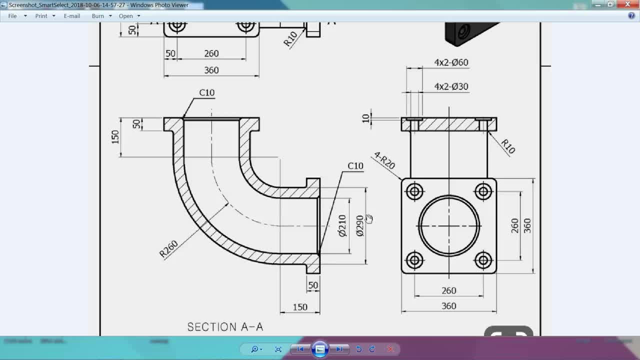 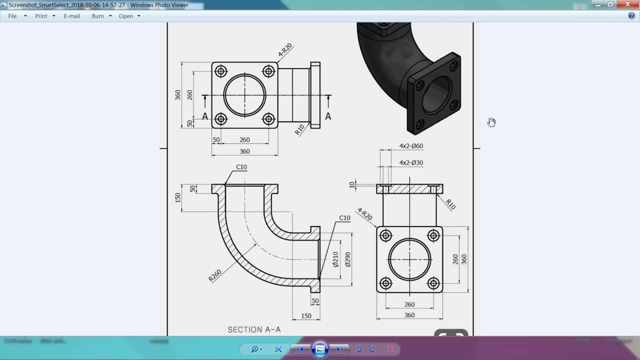 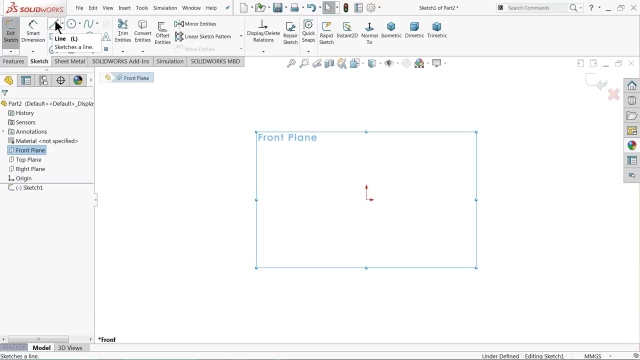 150, 150. And the pipe size is 290. And here shows 210 millimeter. That means the thickness is 40 millimeter. So let's make this one first. Let me choose front plane sketch. Start with line. Draw one line here Now, then move the line. 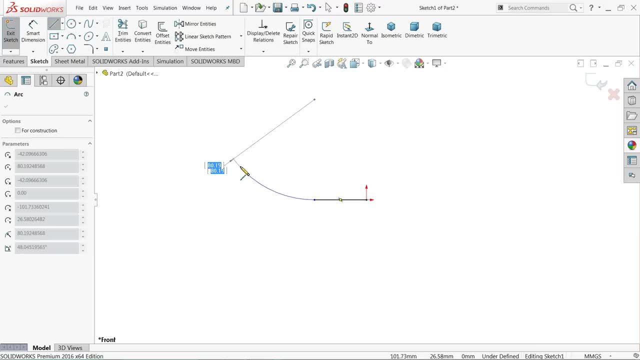 your cursor here, then again go back and see it will automatically convert into circle. once you see it is 90 degree, then click, then drag upward side. exit. now what we will do now. let me choose these two lines: equal relation, that's it. make sure it is tangent relation in both, that's it. let's define. 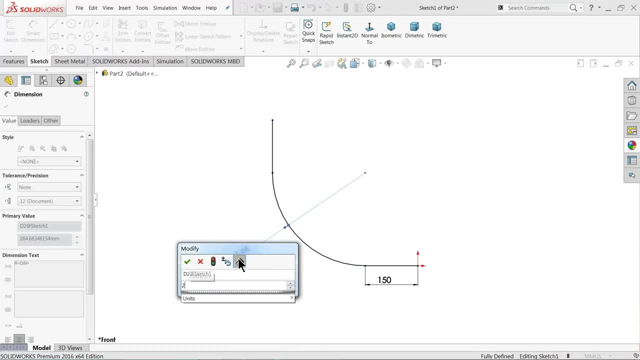 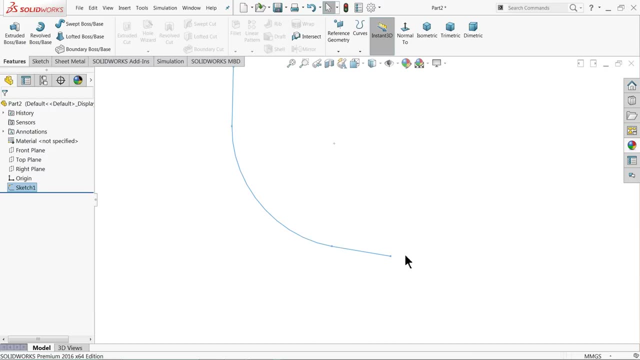 150 millimeter. this radius 260. now see the drawing is fully defined, simply exit. now for creating pipe: we need to create a circular profile, also right plane. it is perfect, just tapered. choose right plane, a sketch circle. now you can see it is a circle. now, if you want to create a circular profile, you can. 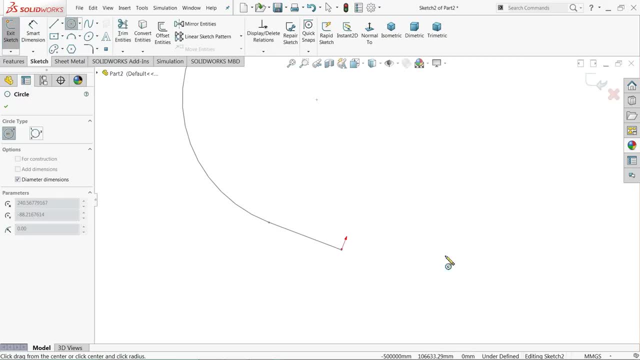 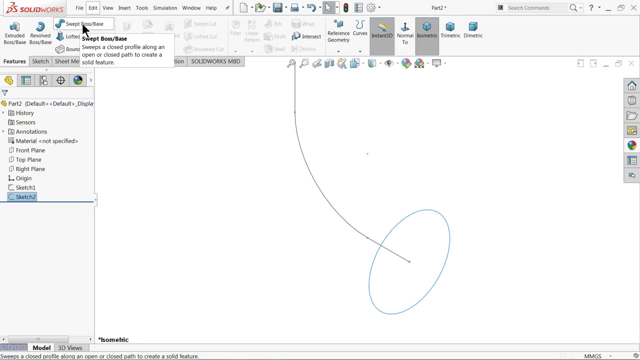 now, this is the point. this is the plane actually where we are going to create a circle. even you can simply select this diameter: 290 millimeter. see now, simply exit isometric view. now just go to feature and choose here very important feature. sweep to boss base command. now here you will see the 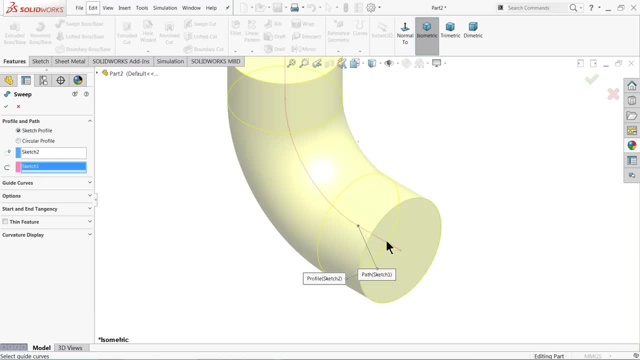 profiles it selected: choose path. so I'll choose here path. but it is going to make a solid, so we need hollow. so what we will do? choose thin feature and thickness: 40 millimeter in. actually, we need thickness inside, so let's keep inside 40 millimeter. okay, that's it. 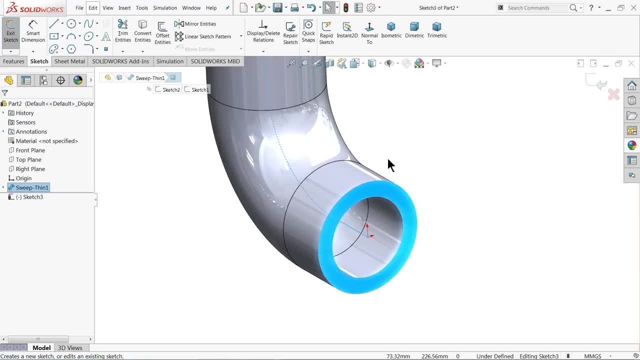 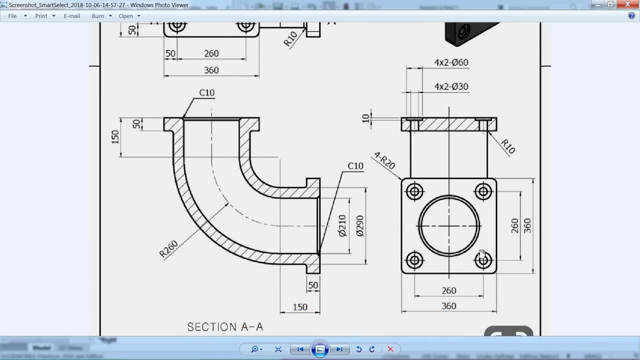 now let me start with flange. choose this face a sketch normal. now see here flange 360 by 360 and the corner radius is 20 millimeter and this flange thickness is 50 millimeter. you will see here and this corner have chamfer 10, so let's get it. 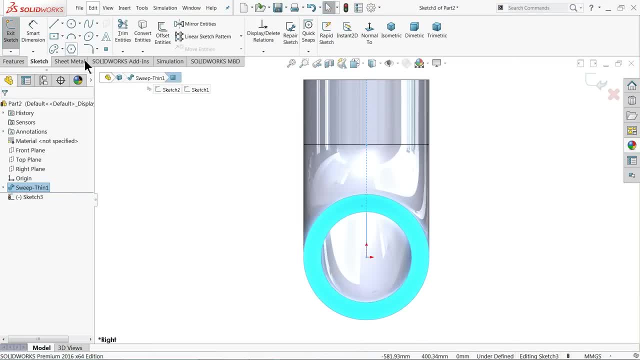 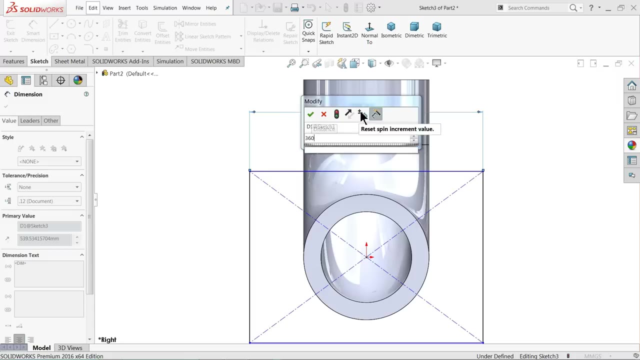 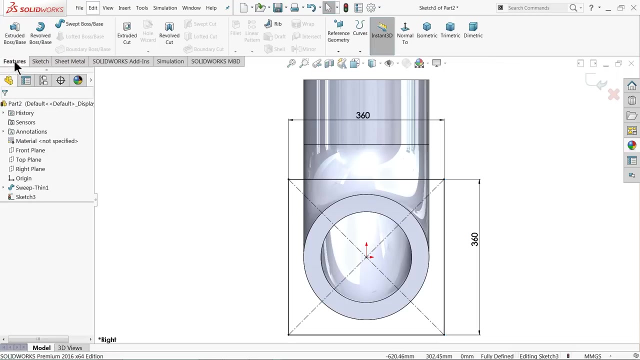 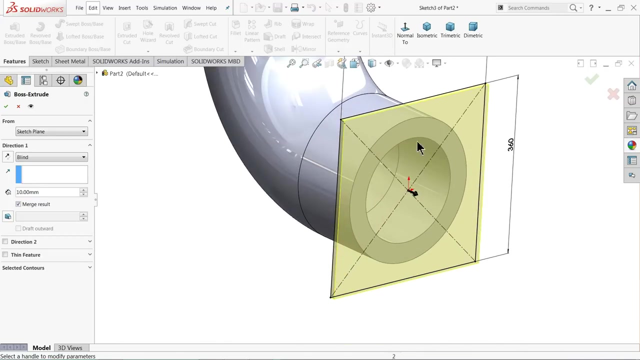 this much. so let's go to this one more time. then I select하는 sample, then next subtley bowl jupiter's combo. go to this littleích, so that's it. so that's it. so let's go to another little box here and let's just click little box Steinbarch. center rectangle and draw one Study Time. нач must have different volumes. ok, so click done. Okay, smart dimension system: 360mm vertical and horizontal, both 360 millimeter. now select extruded or Sorry, extruded boss base, but it's going to be hollow. so what we will do? third, 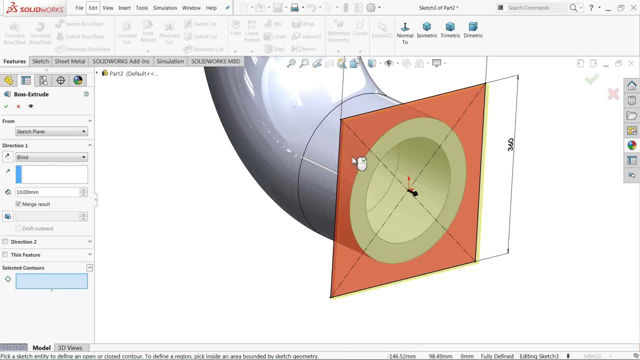 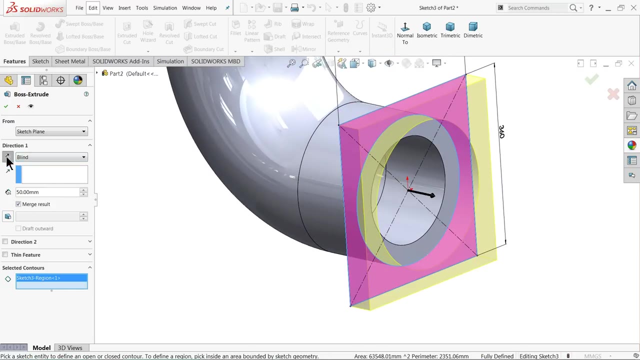 Let me choose here selected contour, So even you can draw a circle also. So we will choose only this. outside face Thickness is 50 mm. It's coming out. So what we will do: Keep here blind Reverse direction. See arrow going inside. 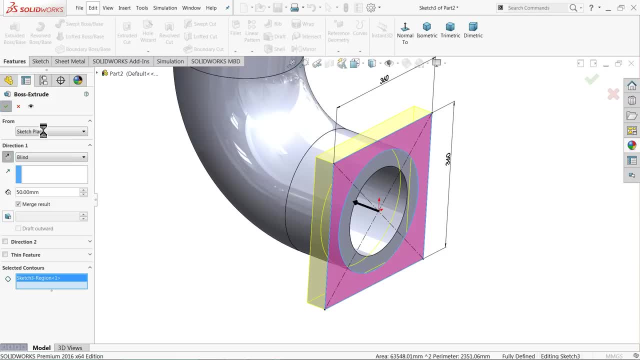 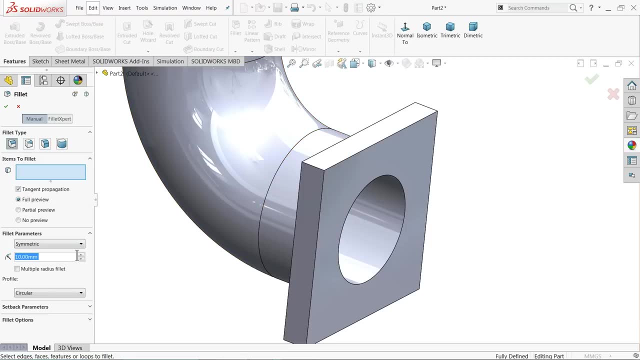 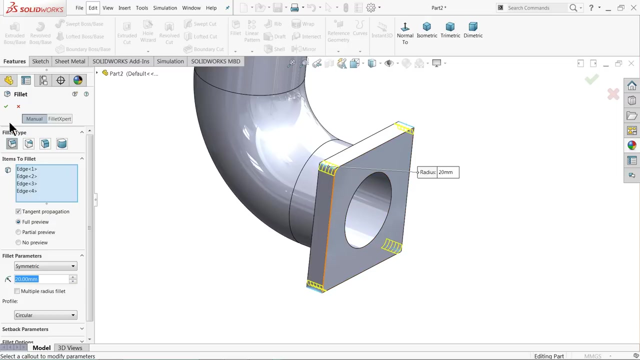 Okay, So this is the extrusion happened. See: Now, fill it. Let me choose. fill it This corner: 20 mm. Choose only one, And here you will see multiple number of small things. Let me select this one, First one, So that it will automatically select all the one. No need to select one by one each. Okay, 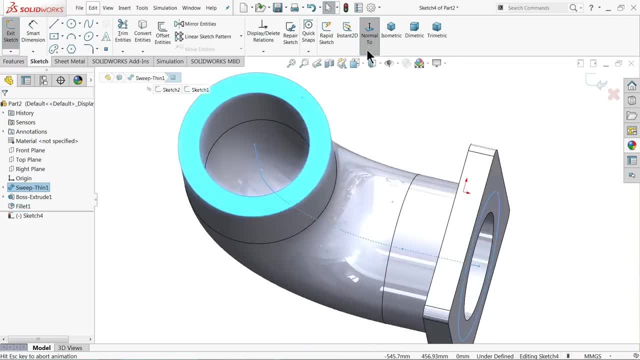 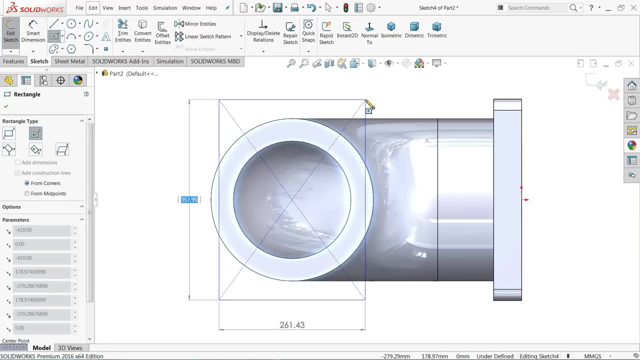 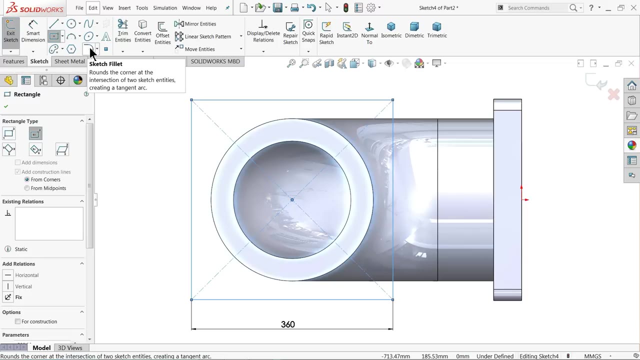 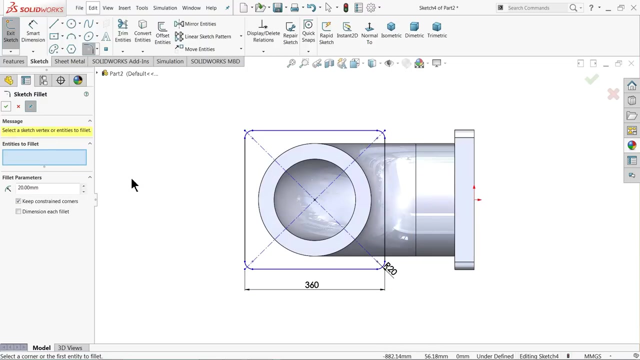 Okay, Now let's perform on this Same here also Opposite direction: Center 360 plus tab key 360.. Even you can simply put here also radius, Select this all 360.. Okay, Now make one relation, This one and this. 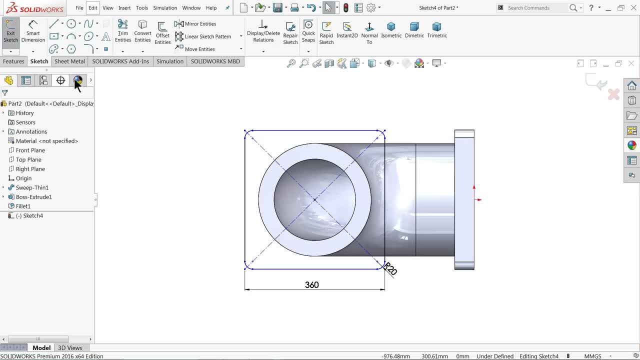 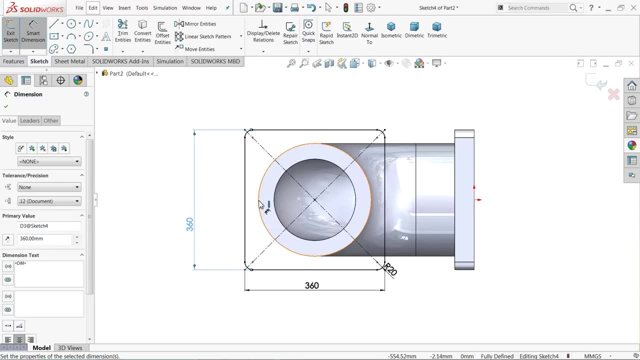 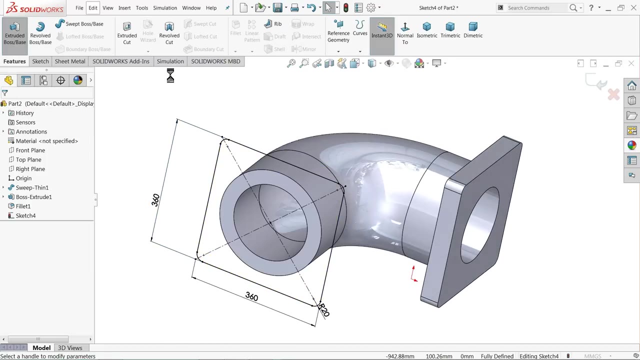 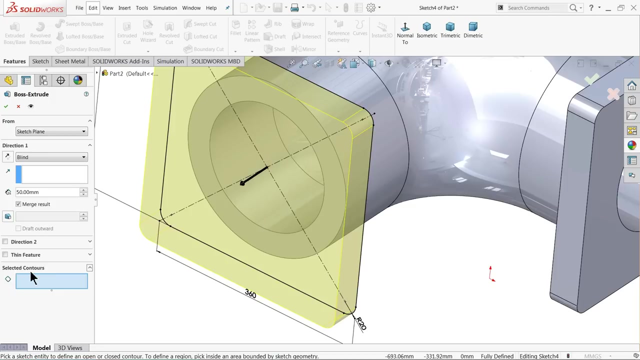 Horizontal Vertical distance. Let's check again. Okay, This one, 360.. Now this drawing, also fully defined, Extruded, cut, Extruded boss base. I forget to Now again the same thing. It's solid. So simply choose here, selected contour And choose outside. 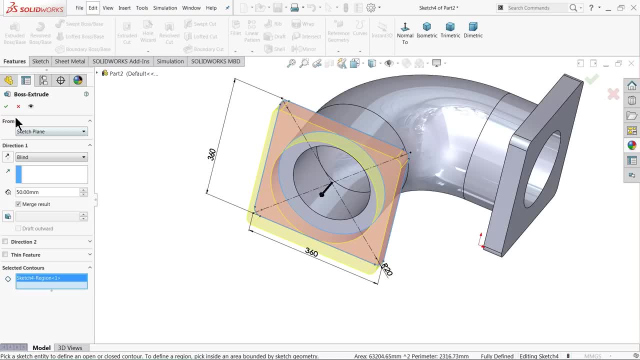 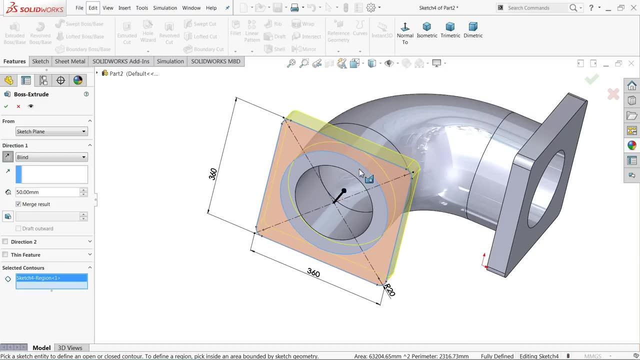 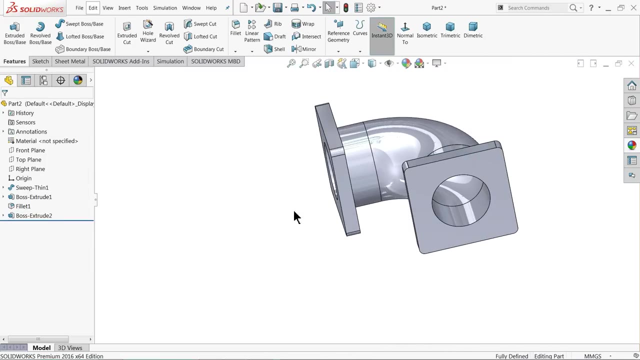 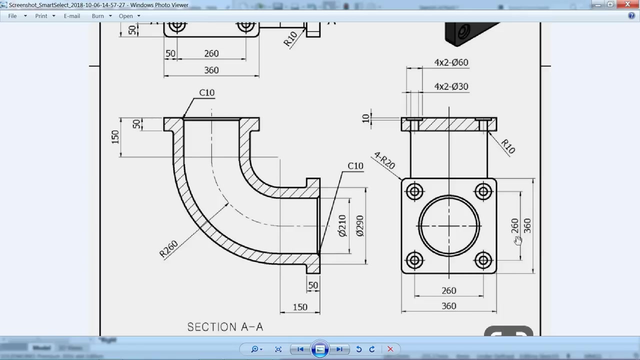 Moving your cursor it will show you where you like to choose. Now it's coming forward side, So 50 mm. Just flip the arrow So that it will move inside. Okay, That's it Sketch. Now let's make this whole. This whole distance is 260 x 360.. And the whole size here: 60 mm, 10 mm. 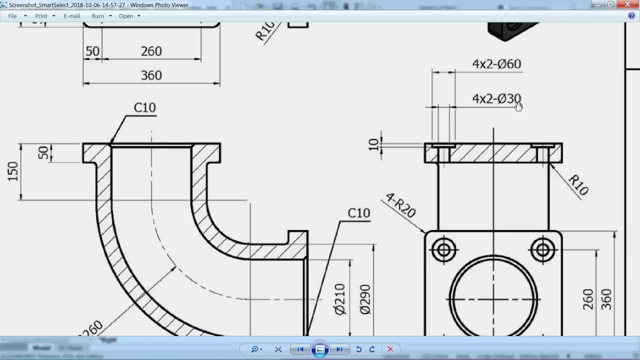 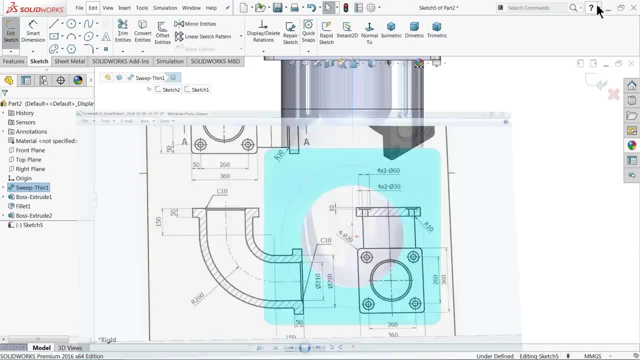 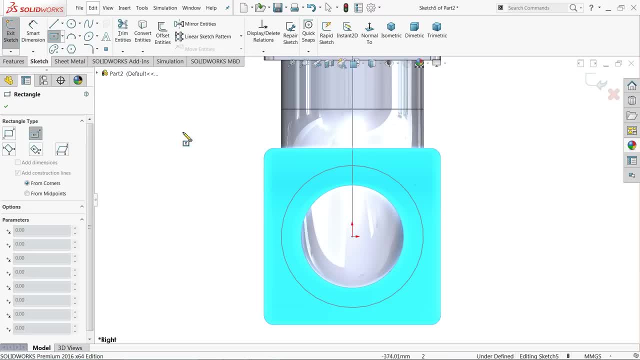 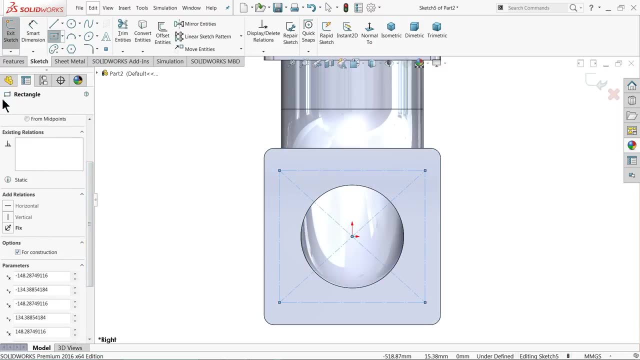 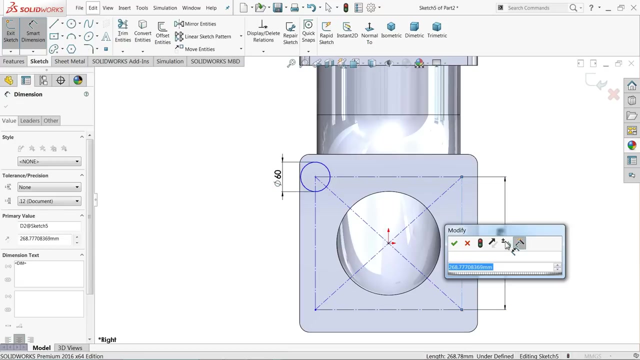 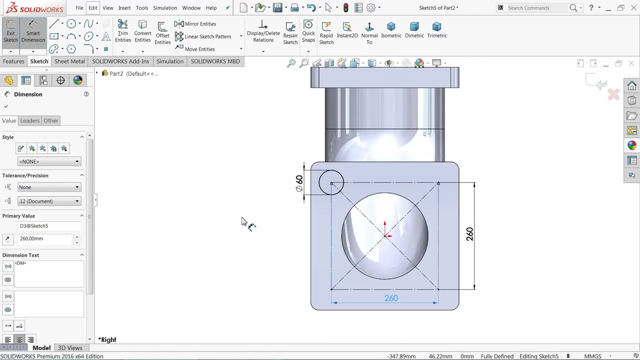 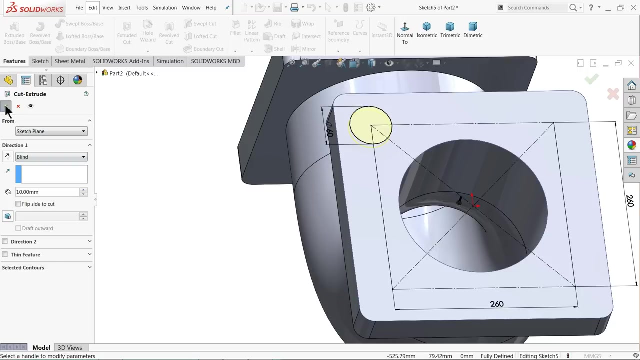 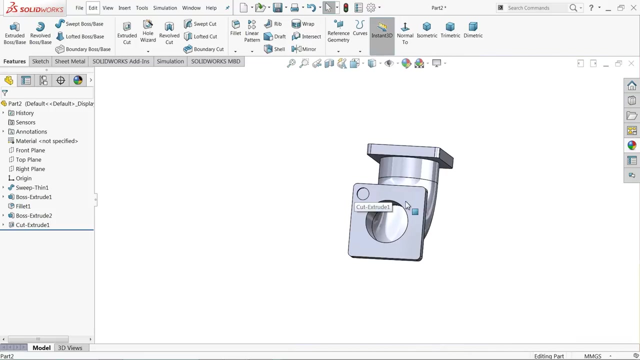 I will choose here center rectangle. No need to choose center. Okay, let's make one center rectangle. Click here for construction purpose Circle And I will draw one circle here and sketch 60 mm, 260, 260.. Extruded cut Now this depth is only 10 mm. See Even. let's. 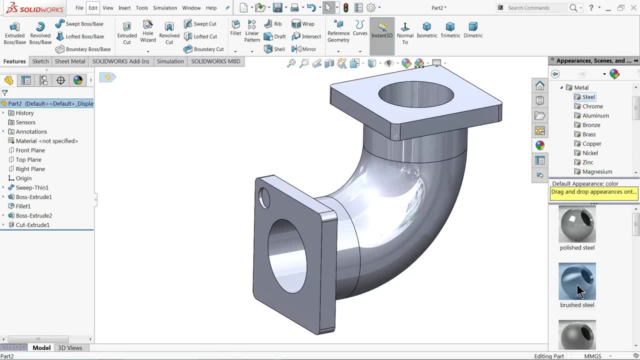 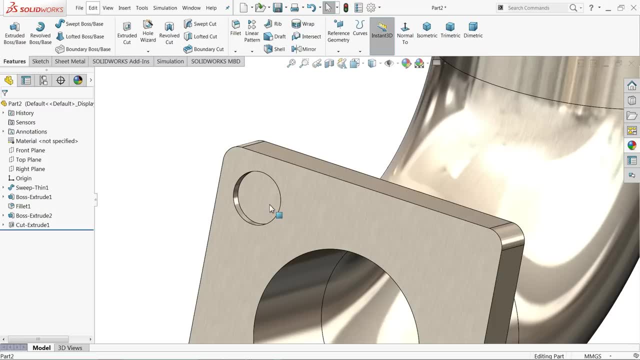 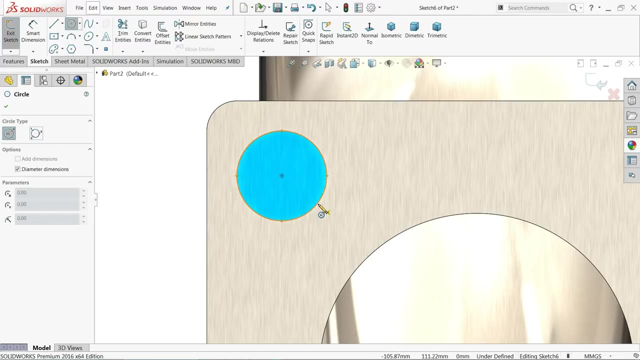 define some material: Steel brushed steel. Nickel brushed nickel. Oh, it's little dark, So this seems better. Now let me choose inside Sketch: normal. Now here we need to make one more throughout hole. Just keep your cursor near to the circle and you will. 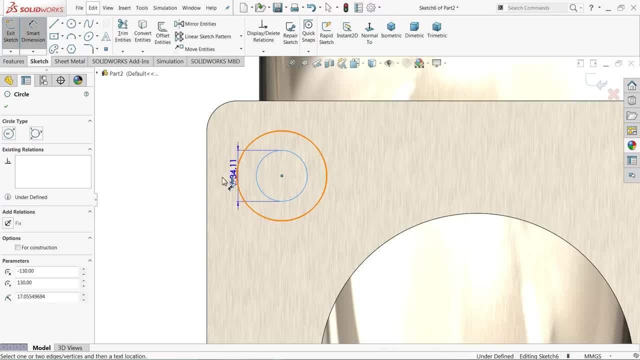 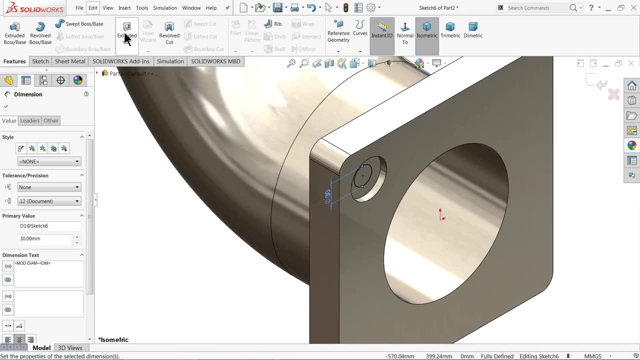 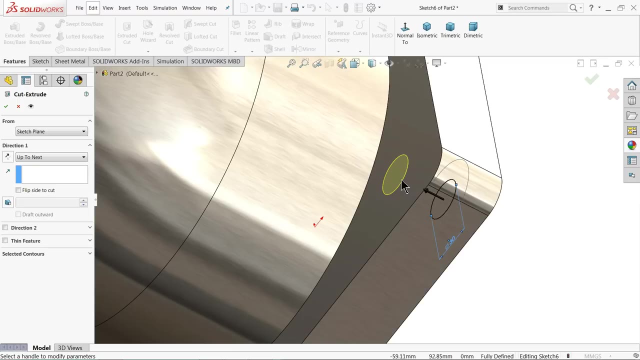 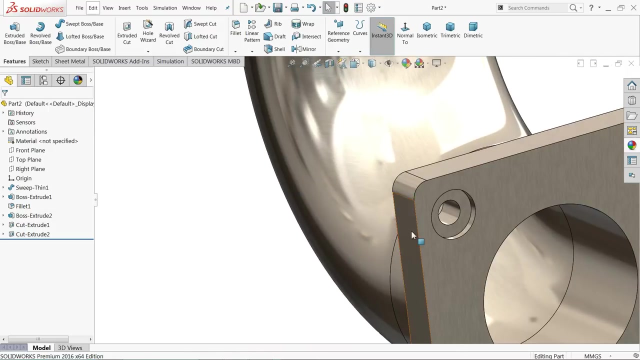 find a center point And, according to drawing, this is 30 mm. It is fully defined, Extruded, Extruded, cut, And we want to cut up to this end. So simply select up to next, So that it will cut up to next face. Okay, Now see, This is how we create it. Now let's make. 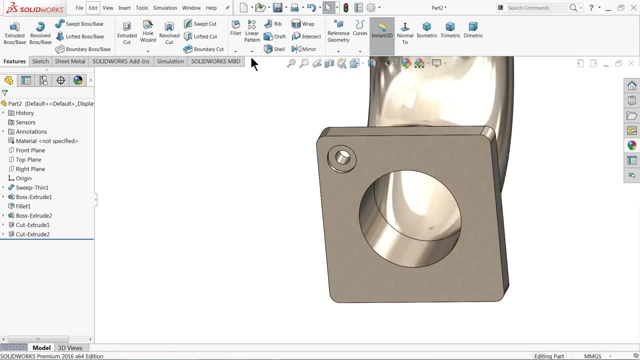 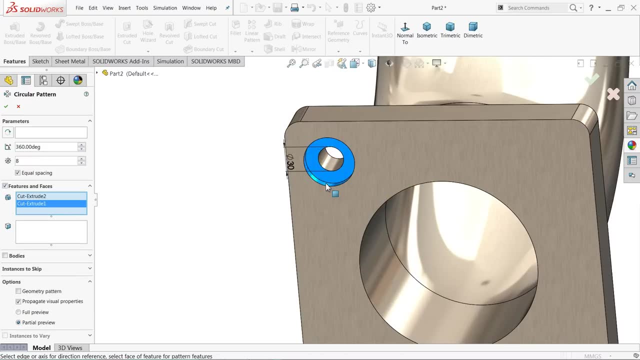 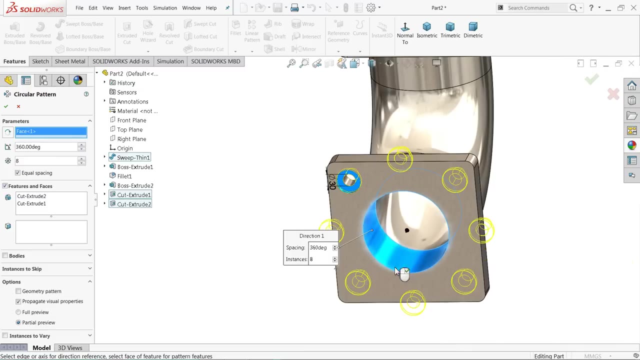 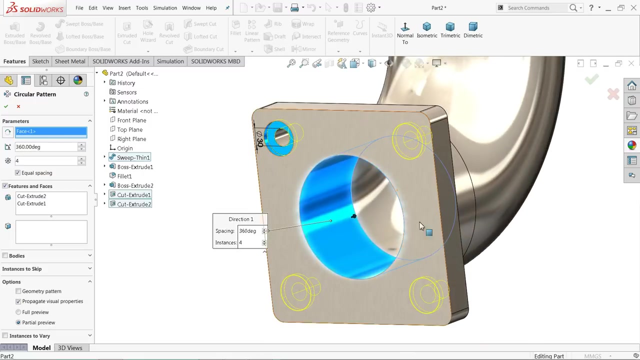 multiple number of this thing. So how we will do this one Now, choose here circular pattern Feature. So select this inside and this one, This too, cut out. Even you can simply select from here. also Select this circular face Equally spacing, and here we need 4 number of patterns. See. 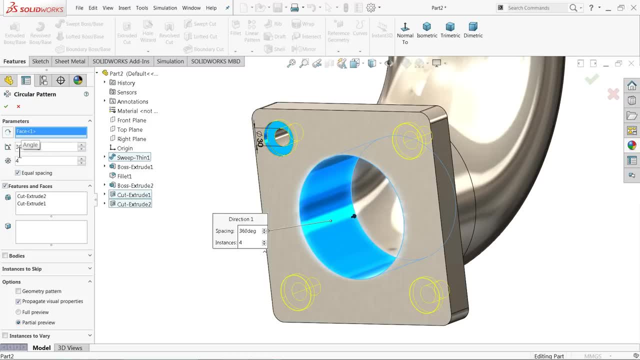 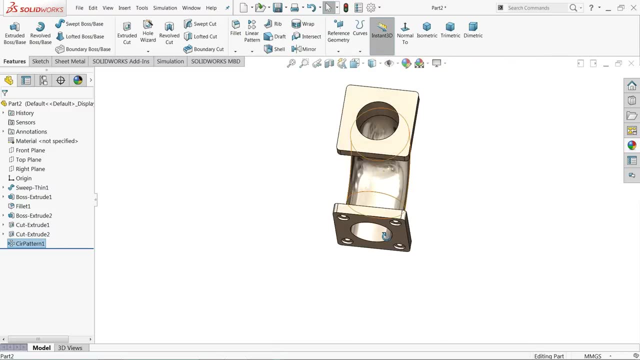 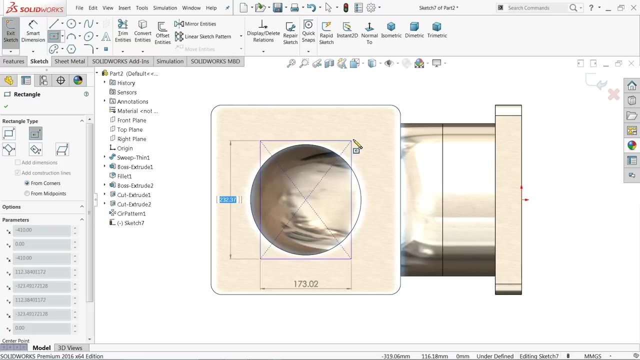 Four. number of patterns: Equally spacing, 360 degree angle: Okay, Oh, that's. look The same thing. let's try here: 260.. Okay, Okay, Okay, 260.. Tap 260.. For construction purpose: okay. 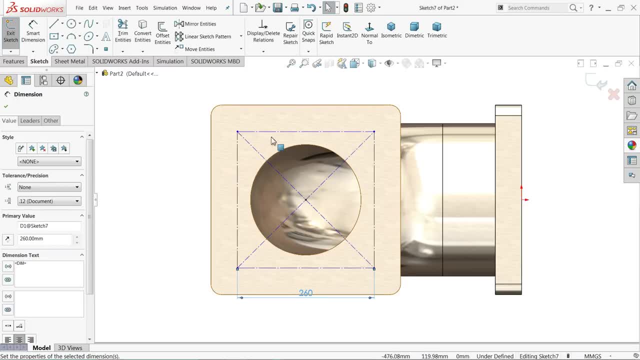 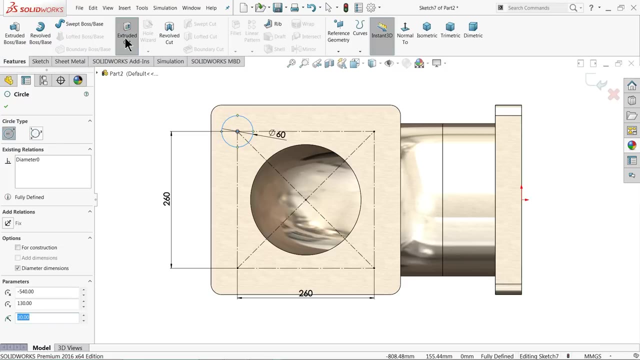 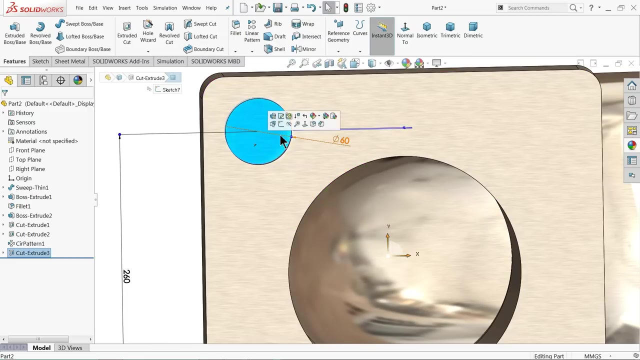 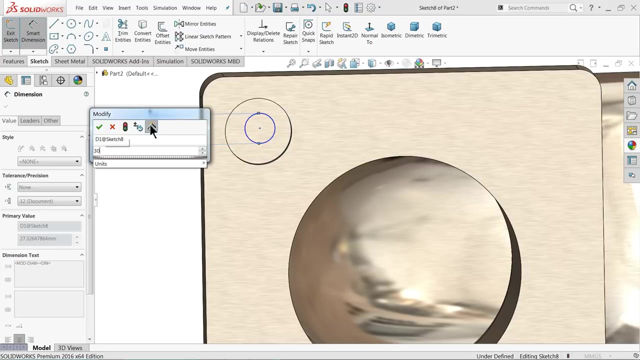 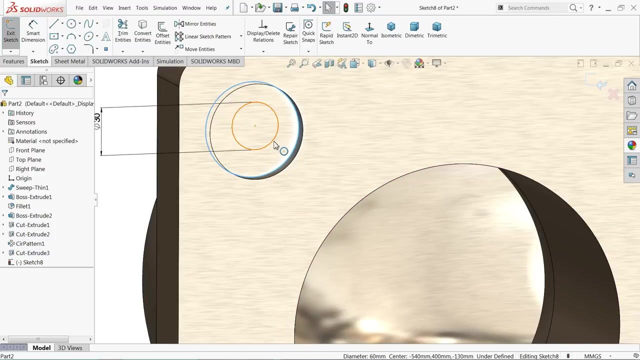 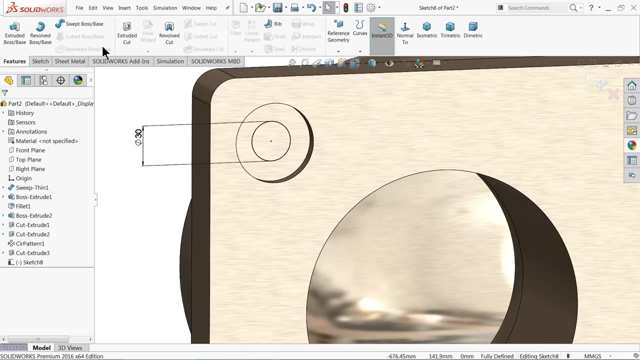 Circle 60 mm. Extruded cut. Keep the depth 10 mm. Now see again. choose the same face. sketch circle 30 mm. Now what we will do: select inside circle and this circle, Make co-centric relation. that's it, so that it will come in center. extruded cut. 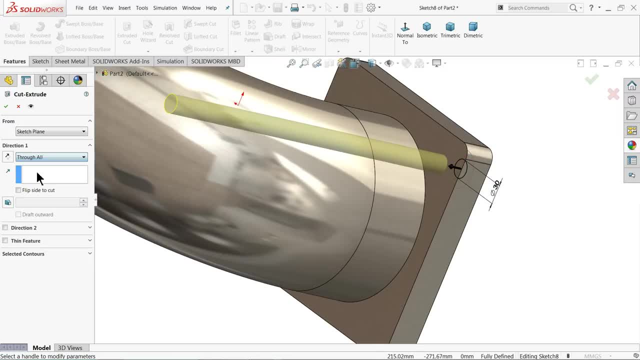 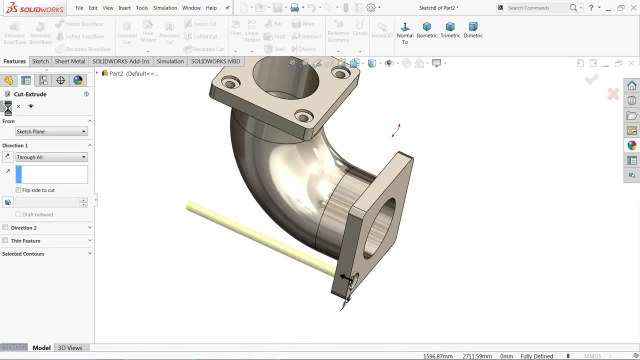 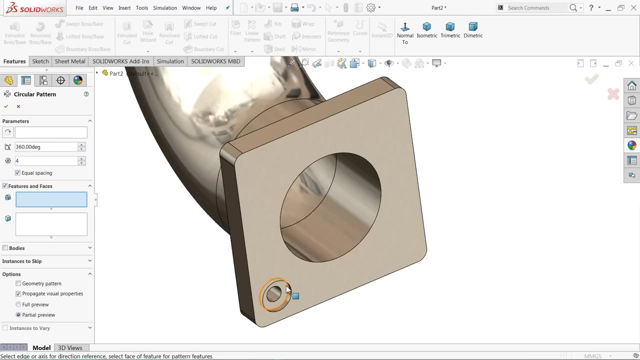 And here you can choose either throughout, see. if you choose throughout, there is chances of attachment. but there is no attachment, so you can keep this also. Circular pattern. drop down this menu: 1, 2, this 2 cutouts and here parameters: choose.